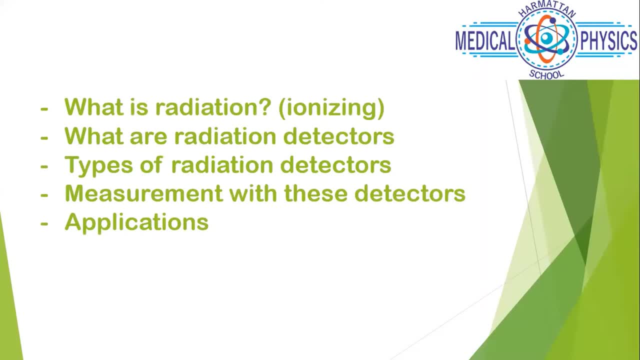 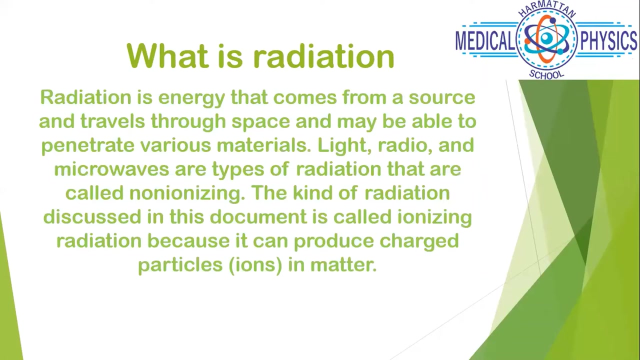 What is radiation? This time around I want to look at ionizing radiation. We also have Non-ionizing radiation. What are radiation detectors, Types of radiation detectors, Measurement with these detectors And possibly we try to look at the application of this detector all around us. So I hope you can hear me clearly. 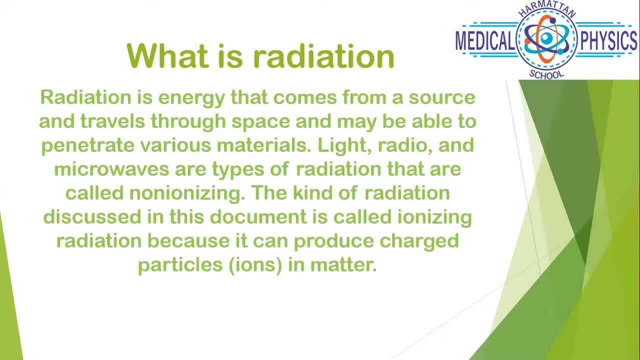 Can I hear you? Fantastic, Yes, we can hear you, please. Good. So what is radiation? Radiation is a material that comes from a source and travels through space and may be able to penetrate various material, So materials like light, radio, light wave, radio wave and microwave. 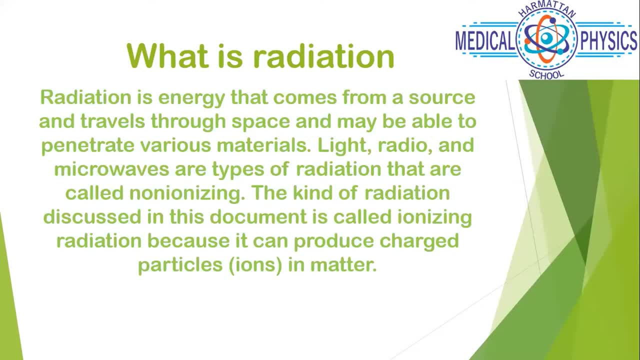 are types of radiation that are called non-ionizing, So they cannot actually ionize matter, So they are non-ionizing. So we likely see excitation. And the kind of radiation discussed in this document is called ionizing radiation because it can produce radiation, So it can produce. 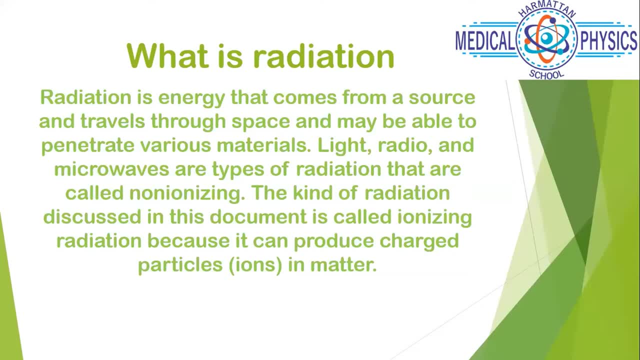 charged particles, called ions in matter. Now I would like to make a clarification here that under radiation detection a simple law plays all through: Ability to produce charged particles, charged ion, electrons and positrons. Now we can from there get images through several. 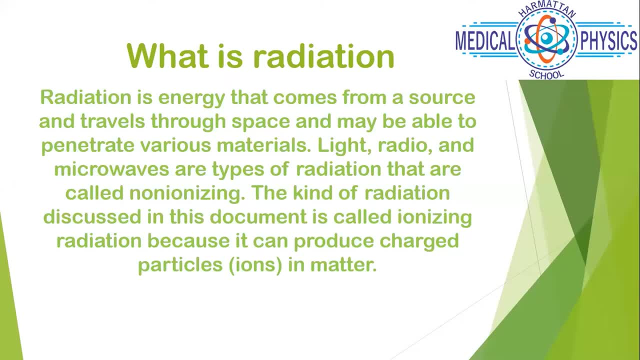 programming languages, through Fourier, Laplace, transform, through whichever means, And then we can also quantify them in terms of measurement, in terms of numbers. So, production of charged particles: it is the main being of most radiation detectors. So once charged particles can be, 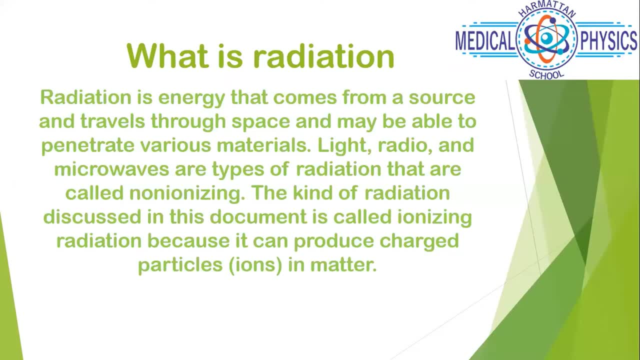 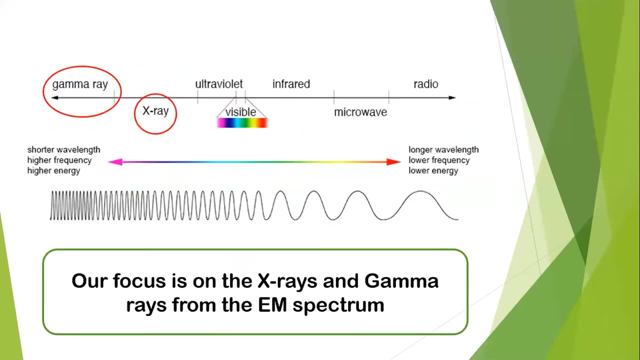 produced. you can be sure that radiation can be measured, images can be gotten. So I think yesterday Prof shared something like this And my other colleagues have also shared something like this. We are particularly about this area, this red area, x-ray and gamma-ray. 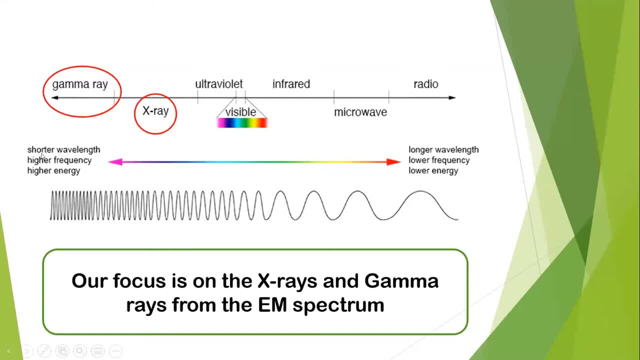 Now we will discover that these particles are actually. they are having shorter wavelength, higher frequency and higher energy, And if you try to look at the other side, you're going to see longer wavelength, lower frequency and lower energy, And this try to tell. 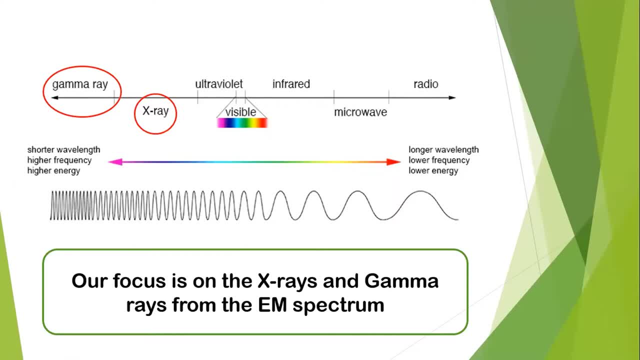 us that you can be in a state and you can be hearing another radio station far away because of the wavelength- very long Now, but in this area we have a very short wavelength because the further you move away from your radiation source, the lower frequency. So that means 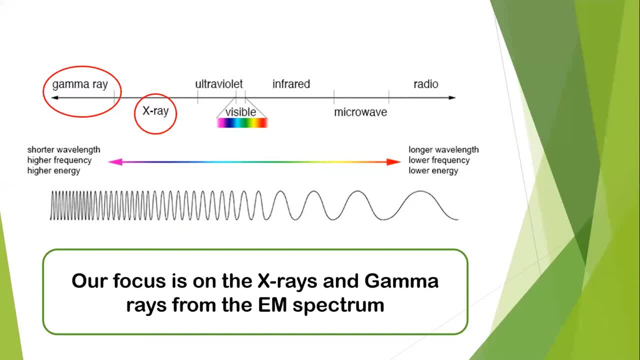 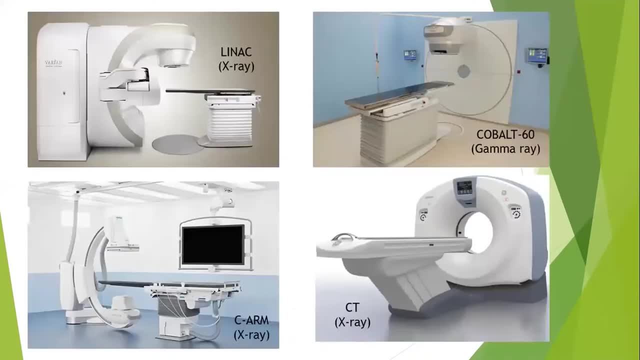 you're going to have much more energy, much more energy, much more heat and much more energy. So the lower the dose. now i'll focus on this, on the x-ray and gamma. our focus will be on x-ray and gamma ray from em spectrum i. i try to just bring out a few device. um, on this side is a linac. 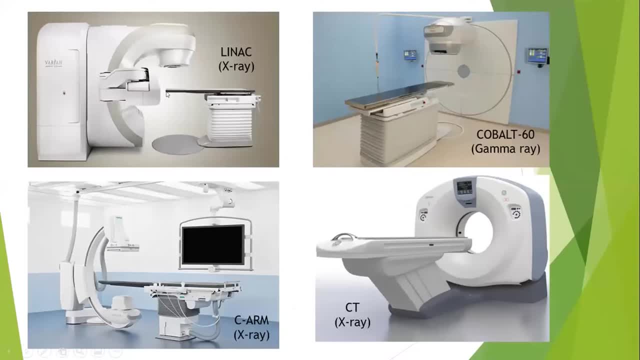 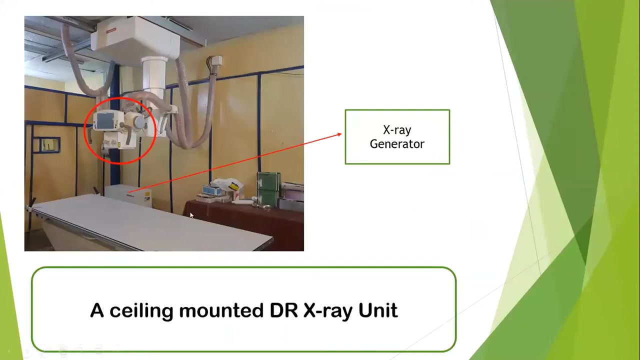 that primarily uses x-ray, high energy x-ray. here is a cobalt, primarily using gamma ray. here is a cm cm x-ray- it's an x-ray. and here is a city- it's also an x-ray. now i i just took this image, uh, from the other lecture. she was trying to show us, um, how an x-ray. 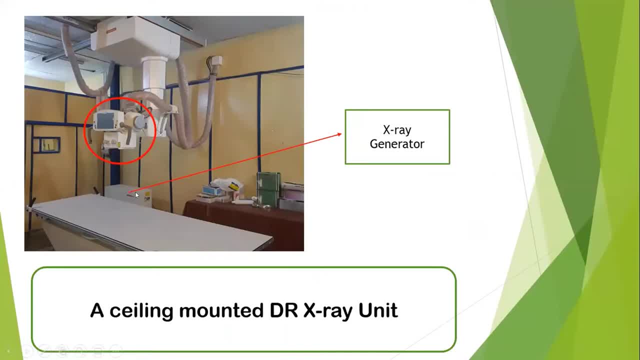 generator looks like we are going to see it more clearly now. the reason why i'm putting all of this is for us to understand this light better when we get to radiation detection and measurement and, um, this area is actually where the x-ray comes out, and these are generator. this is ceiling mounted dr x-ray. 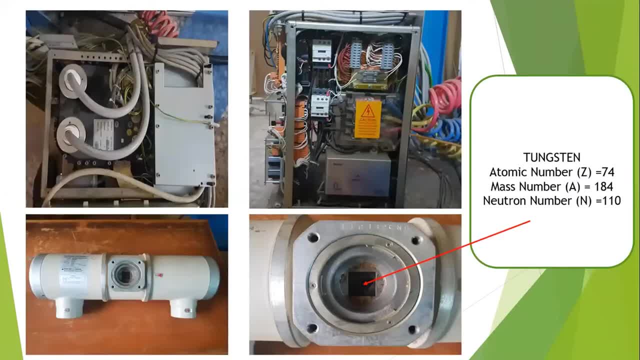 units. now this is what you see on the generator, quite quite um um sophisticated. these are our anode and cartoon. yes, i didn't clarify them here, but one of them is our anode, the other is our cartoon on this transformer. now it's a step-up transformer. 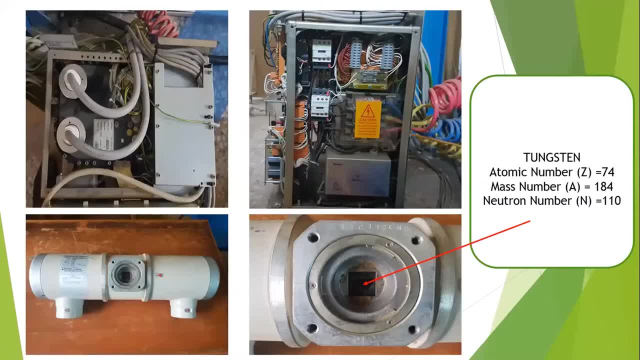 yes, in my country we we operate on 230 volts. now we want to raise this to about 150 000 volts. quite remarkable, and these are the ices of of the x-ray um generator. now we we can see down here an x-ray tube here and um um to a layer of fears most times when we see the diagram of an x-ray tube. 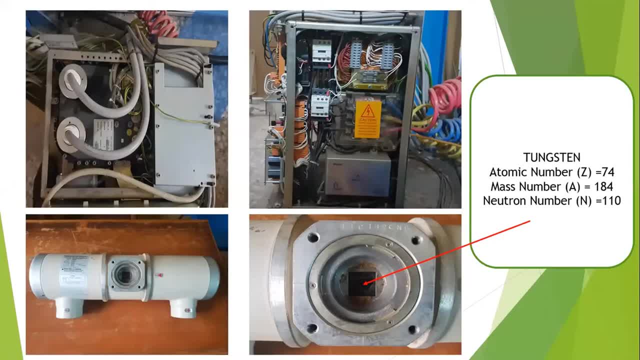 we, we feel the cathode is far and the anode is um quite far. no, they are not. so the cathode is actually the anode, of the anode, of the anode, and then our anode of the anode is actually where i have this red ink is actually our tungsten. our tungsten is just very close. 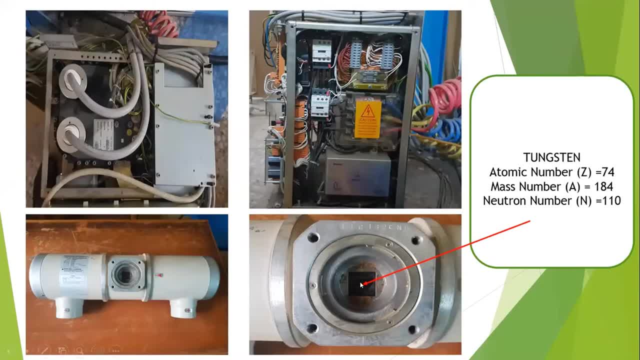 remember, we are seeing very short wavelength, so it's as short as possible. so they are close and they are twined together. we have the anode, and the anode is tungsten, and then we have the tattoo, the cathode filament, where electrons move towards um. 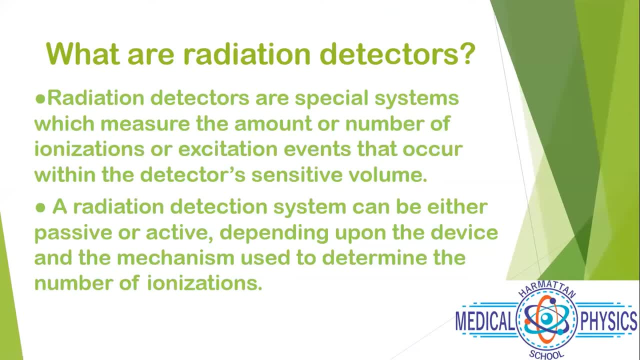 the anode and um um the next slide, radiation detectors. So radiation detectors are special systems which measure the amount or number of ionization and excitation events that occur within the detector's sensitive volume. So now there is a sensitive volume through which measurement is going to be made. 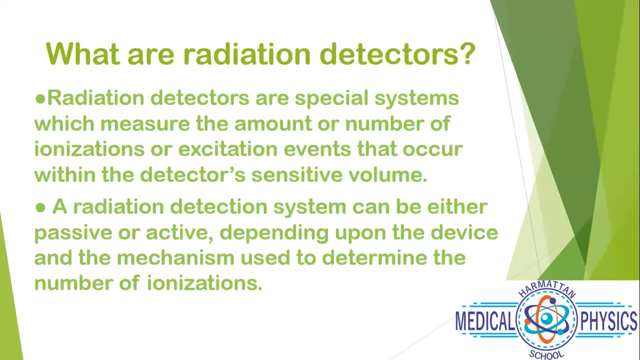 So a radiation detector system can either be passive or active, depending upon the device and the mechanism used to determine the number of ionization. So we are going to look at some of these detectors. actually passive, meaning it has a mechanism for trapping these ions. 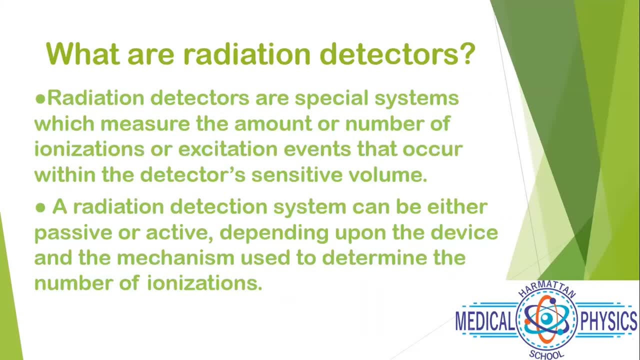 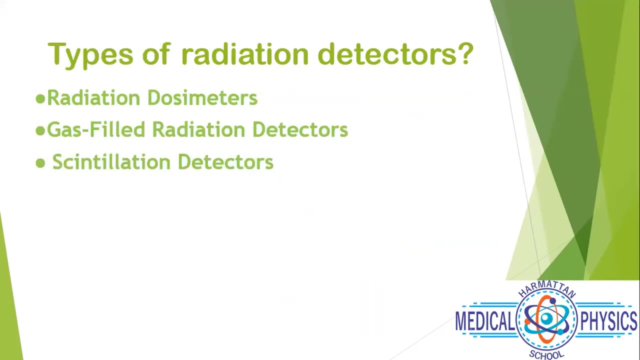 for trapping them somewhere, and then we either heat them up or do something and they are free. So we can now do counting now So active, you get your results immediately, just immediately. So, types of radiation detectors: We have radiation dosimeters. we have gas-fueled radiation detectors. 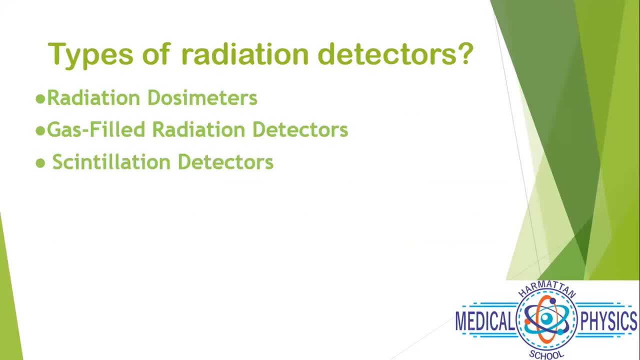 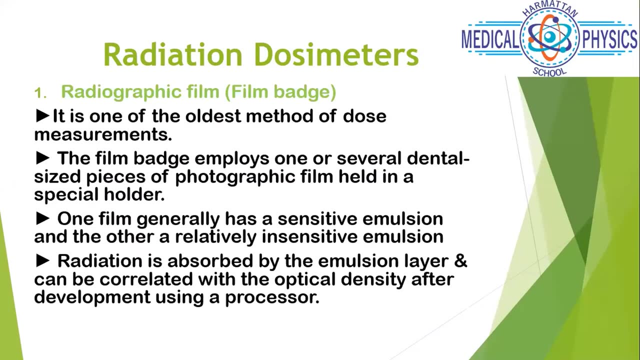 scintillation detectors and I think, lastly, I'm going to add semiconductor detectors. Sorry, it's not here. So one of the first type of radiation dosimeter we use is radiographic films, Which we call film badges. Right from the advent of the introduction of 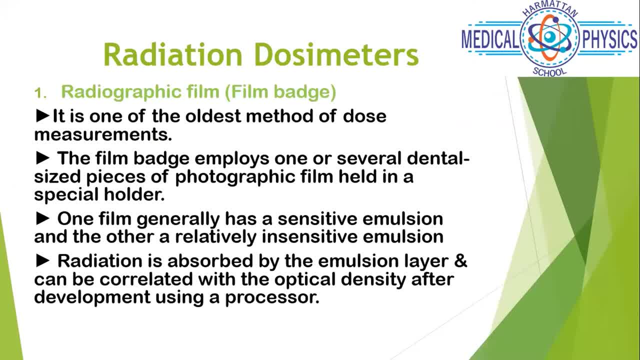 photographic films. exactly, it's just like the photographic film. It is one of the oldest method of dose measurement. The film badge employs one or several dental sized pieces of photographic film held in a special order. One film generally has a sensitive emotion and the other a relatively insensitive emotionally. 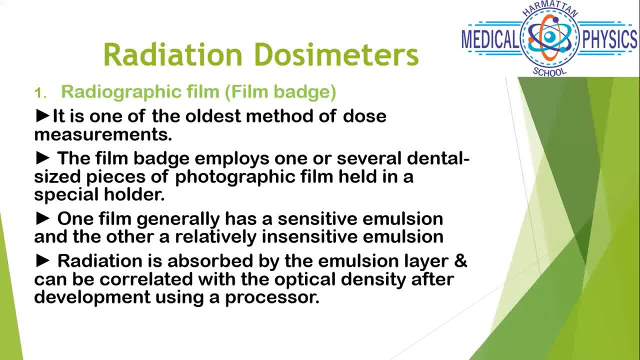 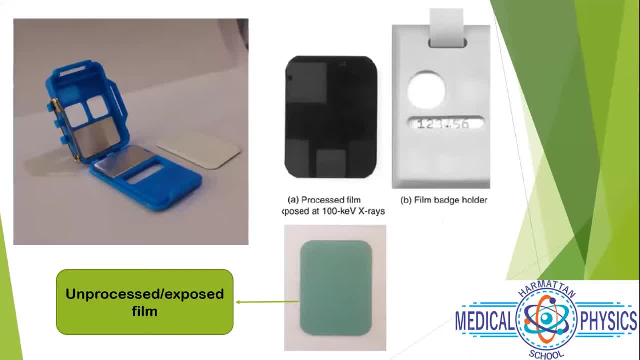 Radiation is absorbed by the emotional layer and can be correlated to the optical density after development using a processor. Now this is actually what we see. This is a processed film. You can see the shades of the grey scale on the film: dark areas, gray areas. 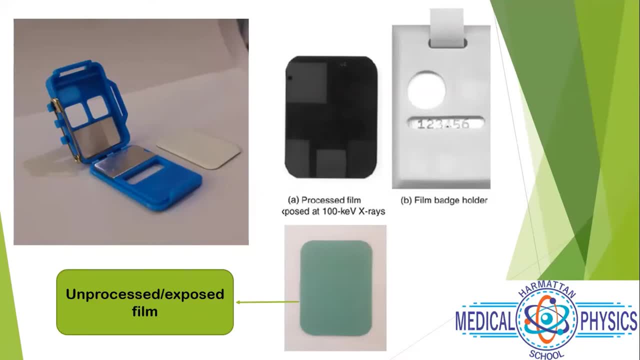 areas and it has to do with how radiation is incident on those areas And from this area. you are going to see this is practically used in the dental department. Go for a dental x-ray. this will be placed inside your mouth using an intraoral x-ray. 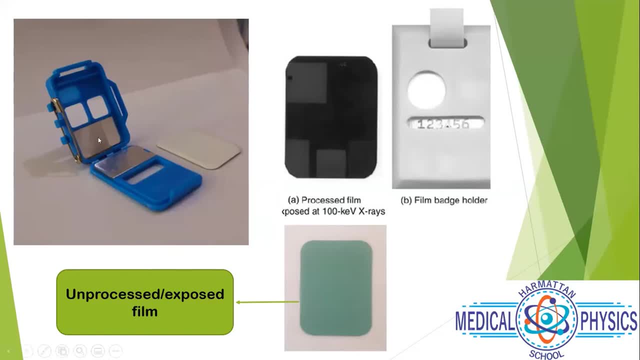 unit, So it's one of the simplest units in that area. So these are also filters. filters are actually attached in order for you to you know when there's a filter blocking. if a filter is used, there's stoppage. 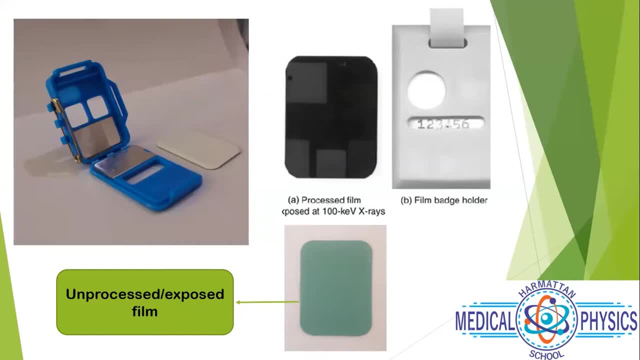 You can have stoppage of x-ray, So the intensity varies with the filters you are going to use. Down here is an unprocessed exposed film. Now I have actually removed it from this point. I actually removed it from here. So this is how the color looks like. 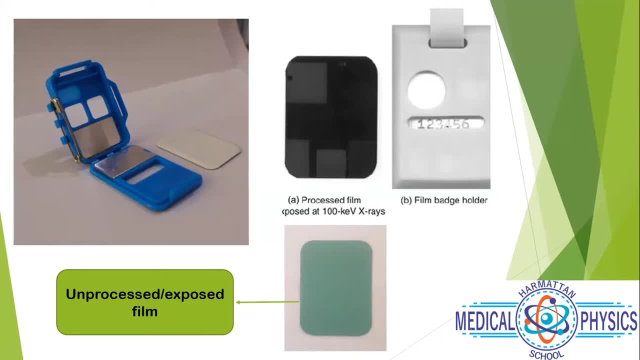 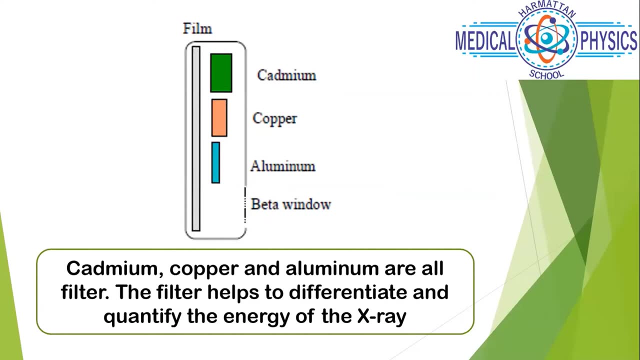 An unexposed- I mean unprocessed, exposed- film. And now this is how it looks. like You can see, cadium. cadium is a bit thicker, copper is relative, aluminum is small. And then this window is quite empty here. 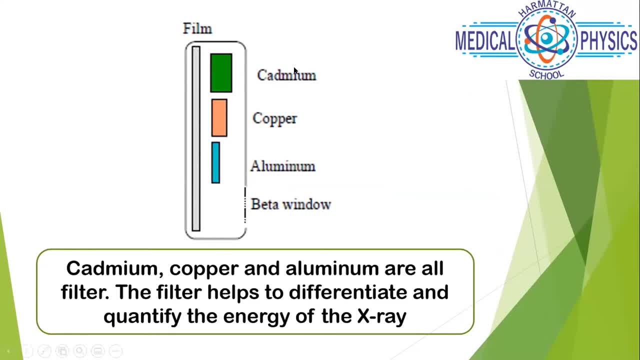 This window is quite empty. The filter will help to differentiate and quantify the energy of the x-ray. So if we're exposing with about 70 kV, you should expect that attenuation. here the cadium is going to attenuate more of the beam. 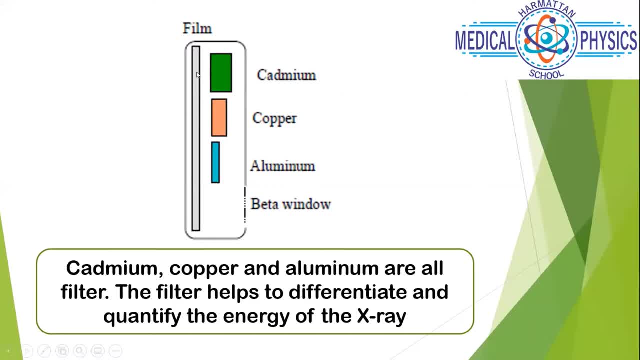 So let us say literally, amount of radiation. So here, Next thing you need to do is: Next thing you need to do is emanating out here For this copper, you have more coming in because the thickness is not as high as this, and in that order. So we actually use this for photographic films. 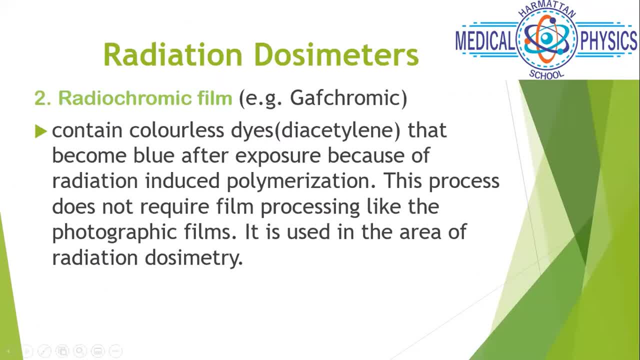 The next one I want to talk about is radiation dosimeters. I want to talk about dichromic films. I don't know whether you have heard of that before. We also call it gaffchromic. They are gaffchromic in nature. They contain colorless dye that becomes blue. 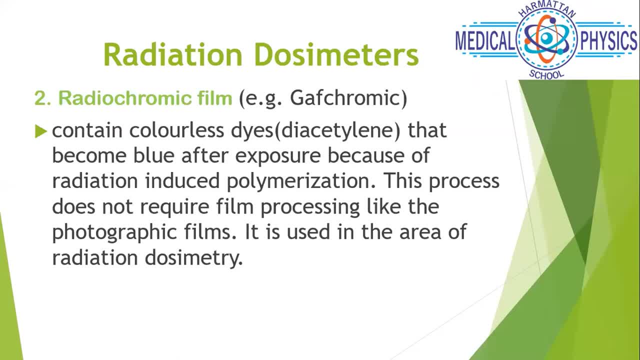 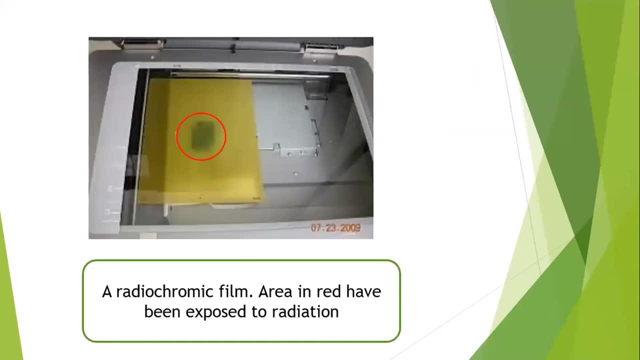 after exposure because of radiation-induced polymerization. So this process does not require film processing. like other photographic films, It is used in the area of radiation dosimetry. You see that we quite use them so much in radiotherapy and other areas. So this is an image of 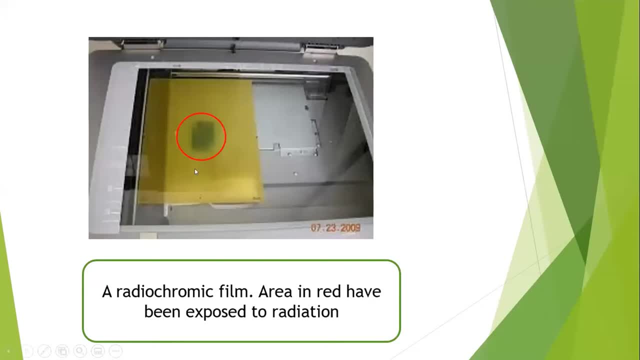 how a radiation dosimeter works. So this is an image of how a radiation dosimeter works. So this is an image of how a radiation dosimeter works. This is what radiochromic film looks like: Yellowish in color, and then you can see the blue areas. 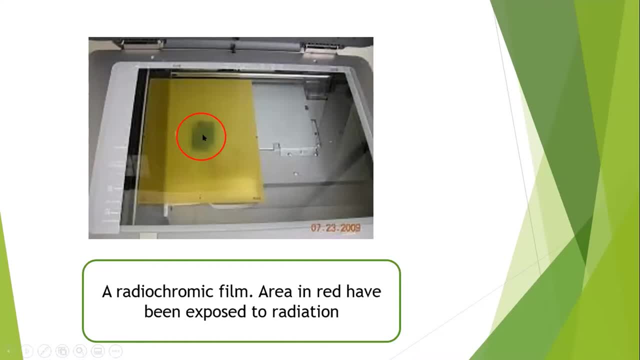 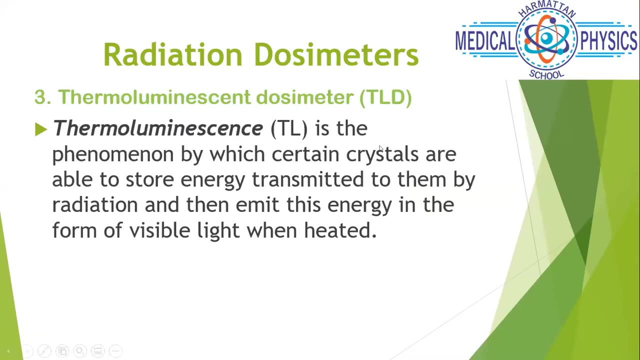 where there is radiation. Now these areas in red have been exposed to radiation, So we practically use a scanner to process our result in this case. The next I want to talk about is thermoluminescence dosimeter. This is quite common and it is readily available everywhere. 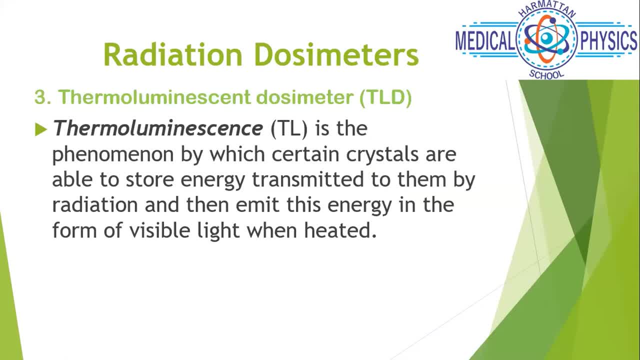 It is the phenomenon by which certain crystals are able to store energy. They're able to store energy transmitted to them by radiation and then emit this energy in the form of visible light when heated. I want to be sure that you can all hear me. Can somebody answer? 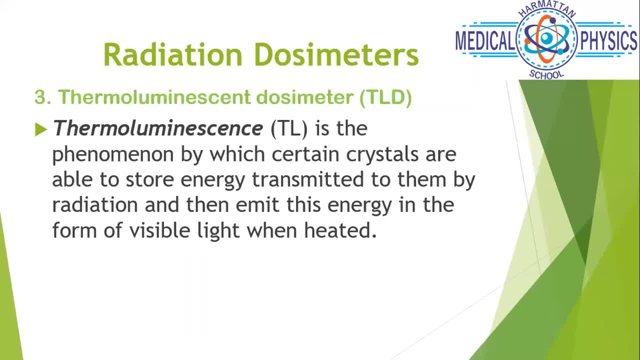 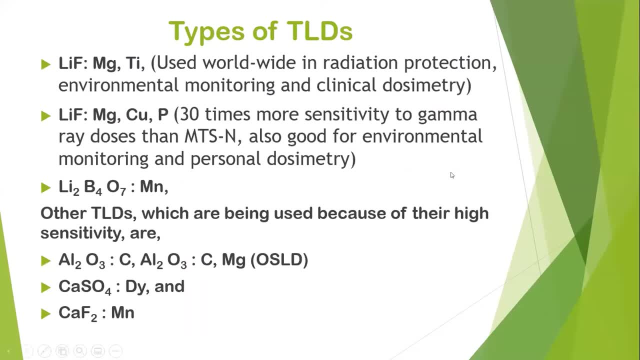 Jessica banquet, Theres andovitch, can you hear кі fantastic, fantastic, fantastic. so we have types of um, tlds, um. the first one is most common: lithium fluoride dupe with magnesium and titanium. now your lithium is actually um neutral abundance. we have what we call neutral abundance of lithium. we also have um enriched lithium, which we call um. 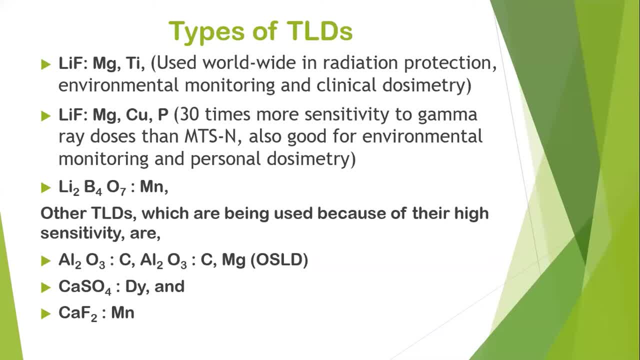 li7, li6. they are all enriched lithium and um we we practically use the first um lithium fluoride dupe with magnesium and titanium for quite a large range: radiation protection, environmental monitoring and clinical dosimetry. now we also have lithium fluoride dupe in magnesium and copper and also 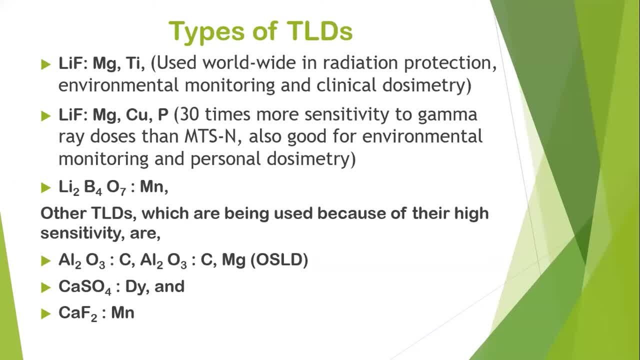 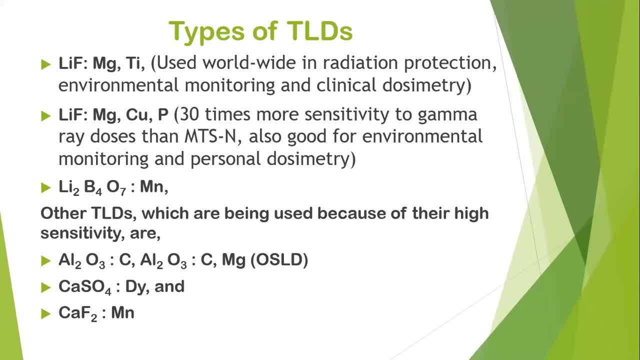 the lithium fluoride dupe with magnesium and titanium, just like the first one um the end is neutral abundance. also good for environmental monitoring and personal dosimetry. uh we, we have a range of them: the family of lithium um. the family of uh, aluminium um. this time around they are also called optically stimulated dosimeters. 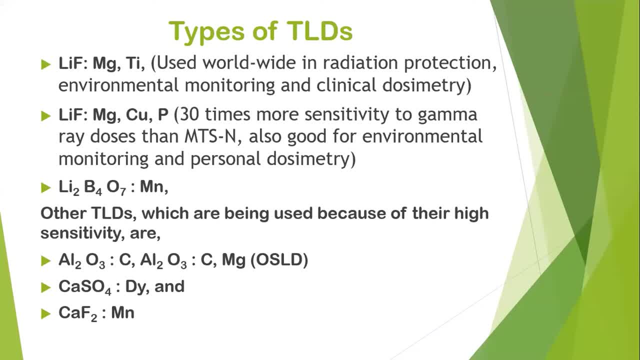 we also have the family of calcium, so they are all practically used for dosimetry. but yes, they actually have some advantages. lithium fluoride, magnesium and titanium is actually tissue equivalent, so most times we use it for uh, patient dose audits. so we can actually use that if you want to, um, find out what your reference dose guideline is for a particular facility. now 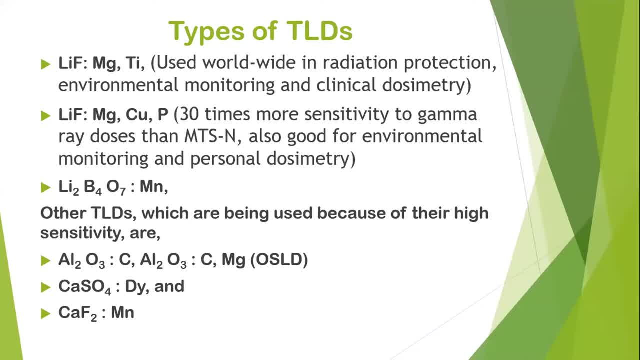 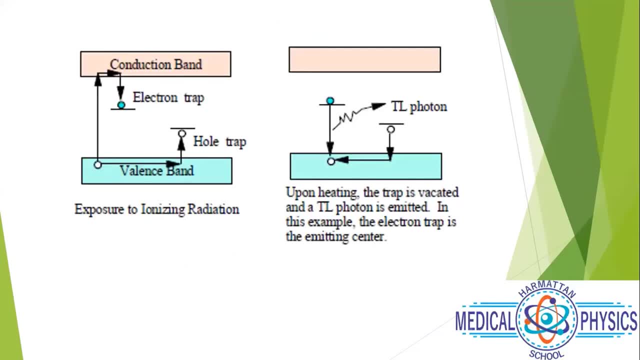 you can also use a lithium fluoride group, the magnesium and titanium, because it is tissue equivalent. um, when you take an x-ray, you don't practically see the um tld there. so, um, this is, uh, the physics aspect of um, um tld and um school physics, um in your part one or your part two. 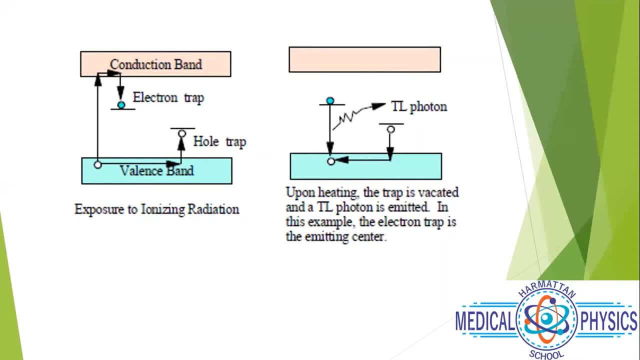 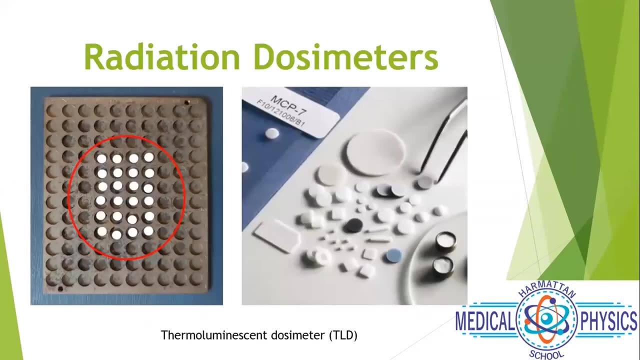 or your part three. you would have seen something like this: your trapped um electrons, your your holes and um your your valence band moving to your conducting band and it's. it's just physics, just physics. so these are dosimeters. i actually took this in my facility um 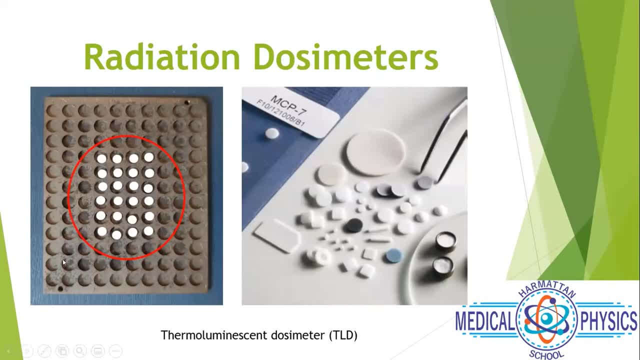 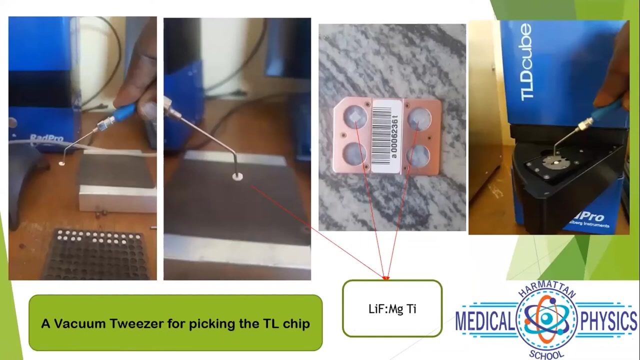 this is a dish that contains 120 chips. you can see them in the um on the tray, and these are different types, quite large. we have them. we have them in powdery form, square in, in round and in cubes, quite large. so i practically had to take this from, uh, our facility. uh, this is a vacuum squeezer. 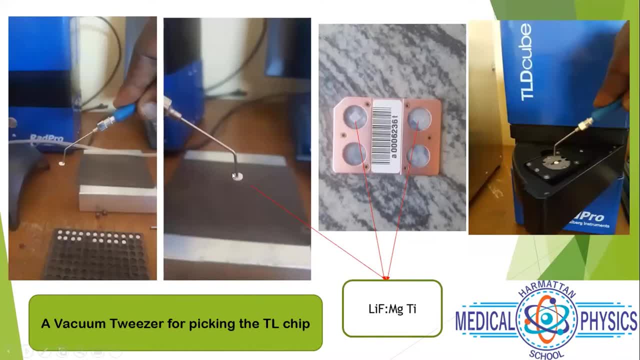 i used in picking this chip from here, you can actually see the thickness of the chip and you can appreciate it more better. so this is lithium fluoride dupe with magnesium and titanium. this is also same. uh, this is another type. uh, you can appreciate them more better and 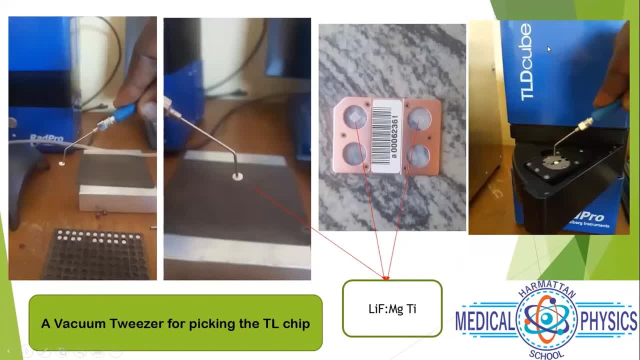 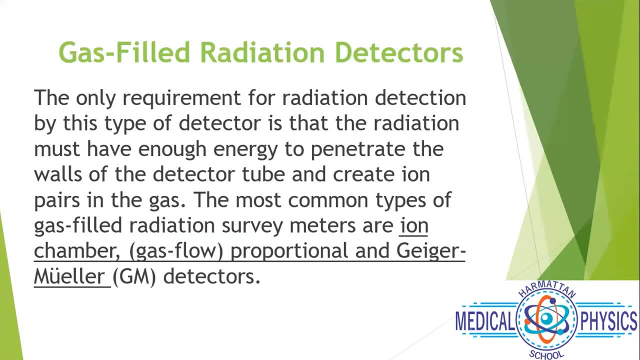 at the rear end. here you can see when i'm i'm trying to load them on a tld reader there for um readouts. so let's quickly move to gas-fueled radiation detectors. i hope i'm not too fast um gas-fueled radiation detectors um the only requirement for radiation detection by this type. 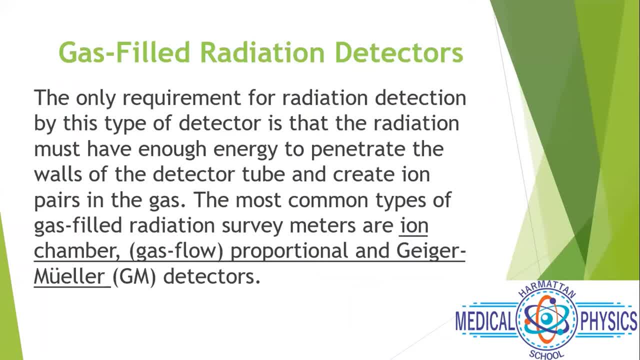 of detector is that the radiation must have enough energy to penetrate the walls of the detector tube and create ion pairs in the gas. so the most common type types of gas, fuel, um radiations of image, um radiation survey meters are the ion chamber, the proportional counter and the gigamolar counter. 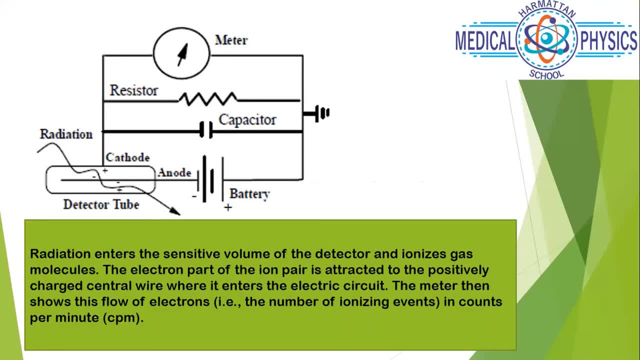 i think that is quite um very clear for us. so this is just um a diagram whereby, um this area is actually the most sensitive area. once radiation comes into this place, there is production of ion pairs. you can see the negative charge and the positive, positive charge. now, from this area, you can 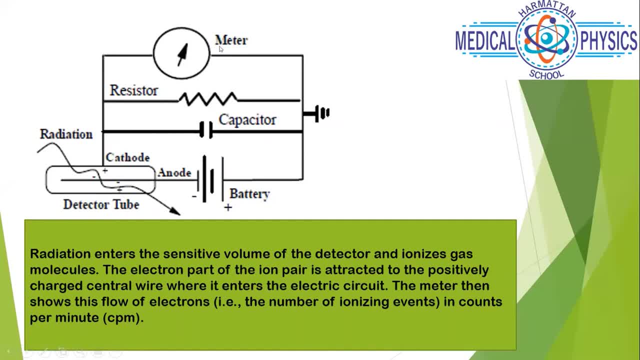 there could be a readout. there could be a readout through some fuel manipulation you could get a a real. so radiation enters the sensitive volume of the detector and ion and ionizes the gas molecule. so the electron part of the ion is attracted to the positively charged central wire where the entire when the way it enters the electric 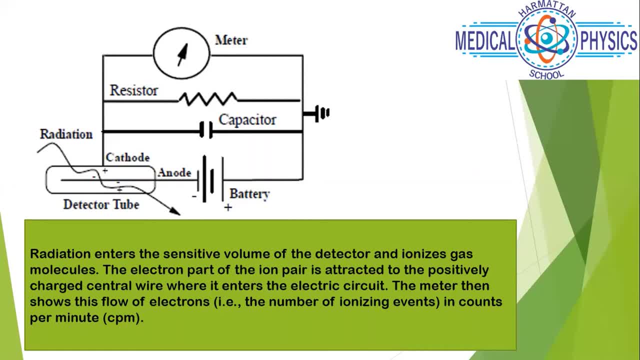 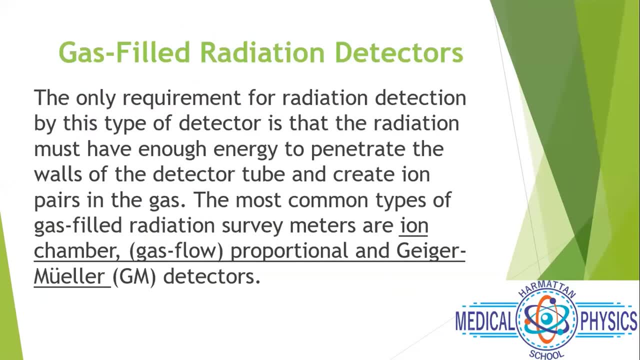 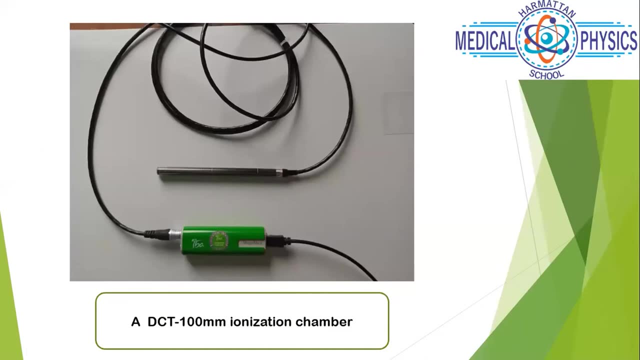 circuit. so the meter then shows this flow of electrons. so it's quite um easy to measure. so i i want to show you um an ion chamber. so this is an iba ion chamber, a dct um 100 millimeter ion chamber. when i talk about the length you learn from here down here and then 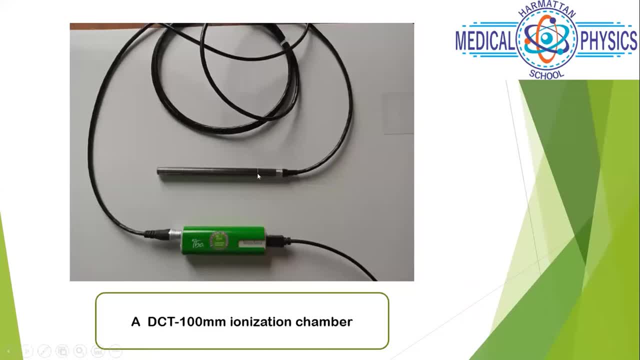 it has a sensitive area. here we have the sensitive volume um. you can actually use this quite expensive um for um those measurements we will. we usually use this for um those measurements for ctdi. you know you want to get your your um, um, you want to get your dose output using your. 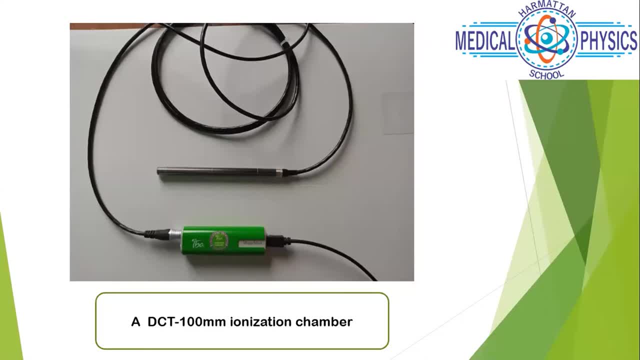 16 centimeter um, um, um phantom, um, and your um 32 centimeter, um um phantom. you want to get those at um 12, or 3 at 6, at 9.. so we can actually use this for those measurements and um, um. i quickly moved to proportional counter. 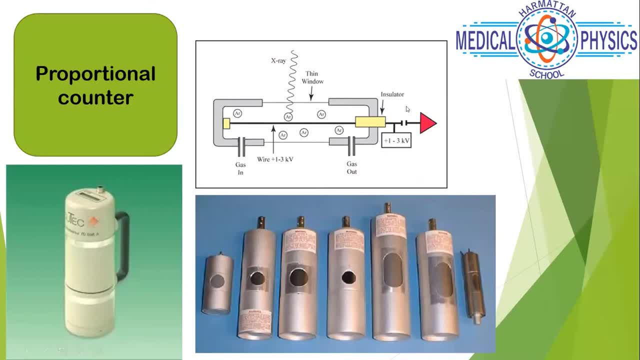 it's um, it's um. it uses the principle above. here you can see the team window. you can see the ionization of the argon gas here, and it's just purely ionization. so once ionization can take place, charges can be collected. now these charges can be converted into numerical values. 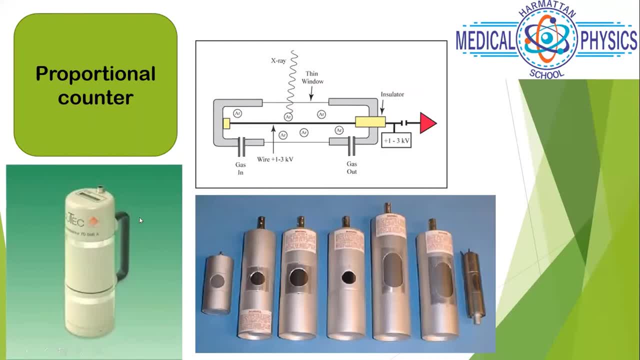 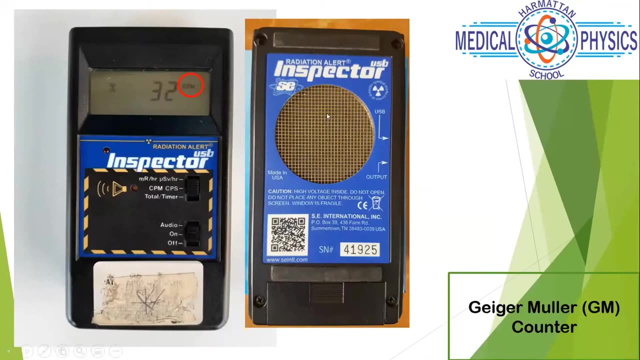 they can be converted into numerical values. so this is an example of a proportional counter, and they're a bit bulky and you don't often see them. so i um this is a gigamolar counter, um, very straightforward, um, you can see, you can actually measure in, count per minute. 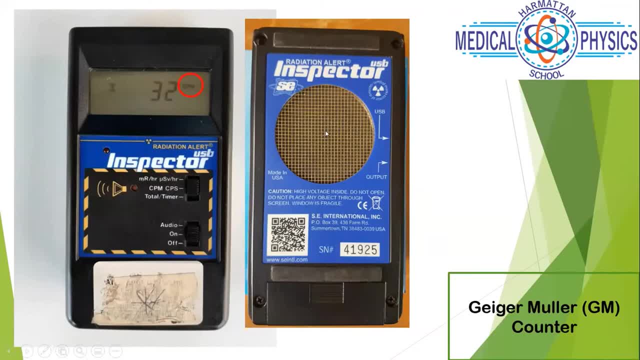 uh, this is the sensitive area. this is the sensitive area. as you can see. you can measure a millirouge per hour, microsievert per hour, count per minute, count per seconds, so you can do a range of measurements using this gigamolar. same thing there is: ionization: charges are collected and they are displayed in form of numbers. so i 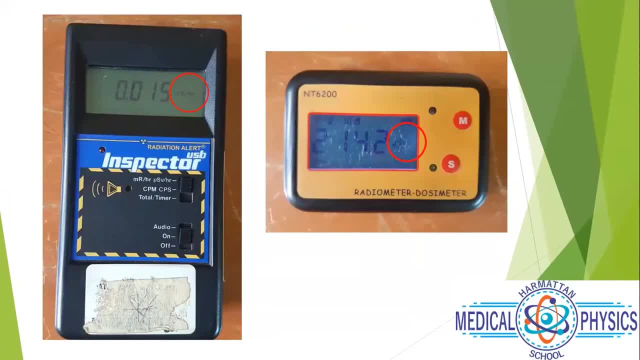 have a range of them. uh, we have um, um, it's also displayed in millerogen per hour. this is it, millerogen per hour. and this is another type of armory: um meter that can also measure in microsieverts and in terms of equivalent dues, and we can also measure in, uh, those rates, so you can get full range of that. 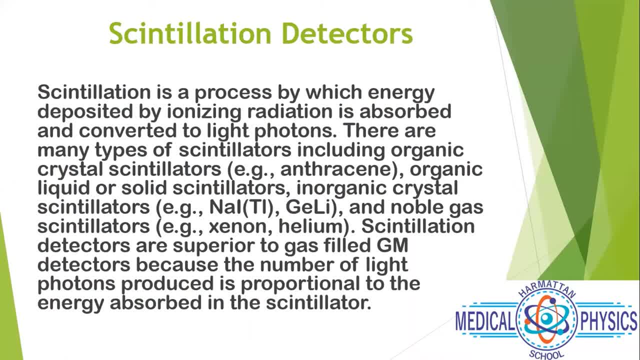 so we quickly look at scintillators um now. um, scintillation is a process by which energy- energy deposited by ionizing radiation- is absorbed and converted to light, so there is a conversion to light. there are many uh types of scintillators um, ranging from organic crystals and inorganic crystals. 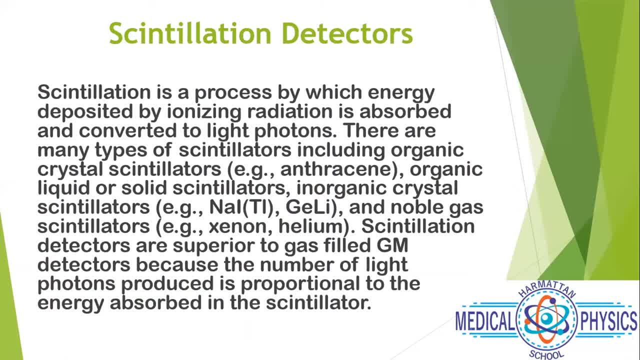 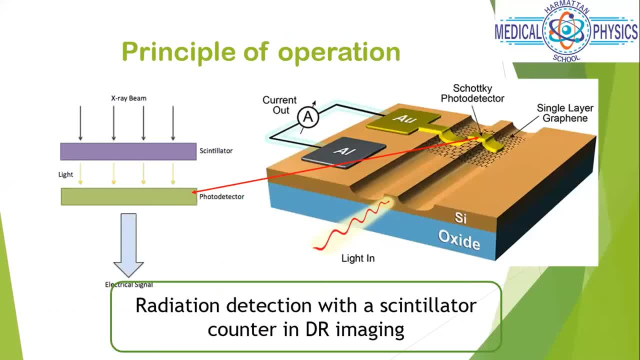 so common to us are um the sodium iodide. uh are dealt with um thallium and we have xenon, we have helium gas. so this is the principle of operation. quite dramatic here, a lot of physics here. you would have seen this in your solenoid's prism. but when the51- door trap grabs youいや sp moves your. 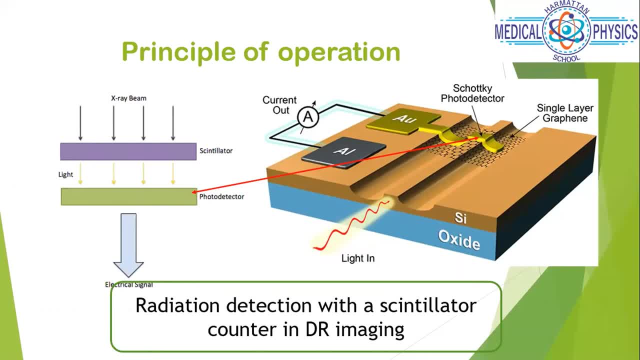 state, um, uh, possibly we'll get there a bit in your solid state physics. now we have x-ray incident on the scintillator. now the scintillator has the capacity, the strength to give out light, and this is just light. now the light goes through a photo detector. now i have drawn here. this is a photo. 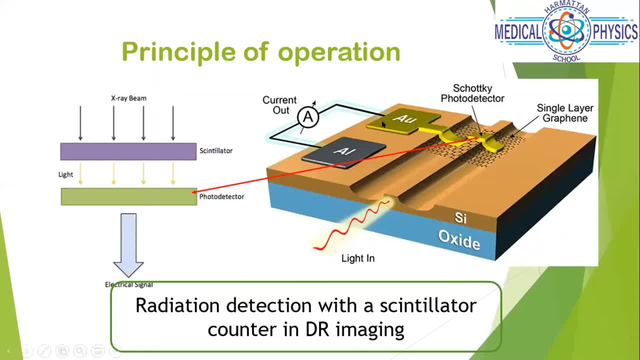 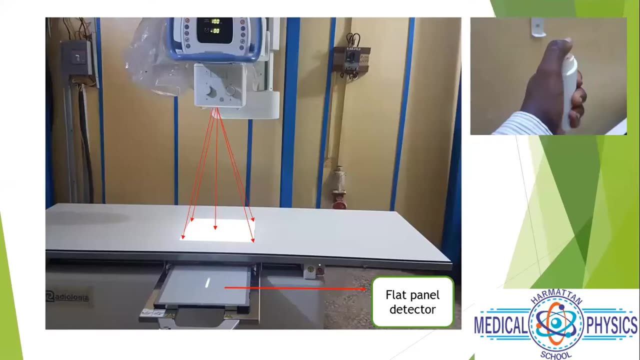 detector, the photo detector um, is actually to help us to combat this light to electrical signal. quite amazing. i, i, i use the dr system here for that. um, one of our dr system. if you have heard of a flat panel system, here you can clearly see- sorry, let me move my cursor here- so this is a flat panel. 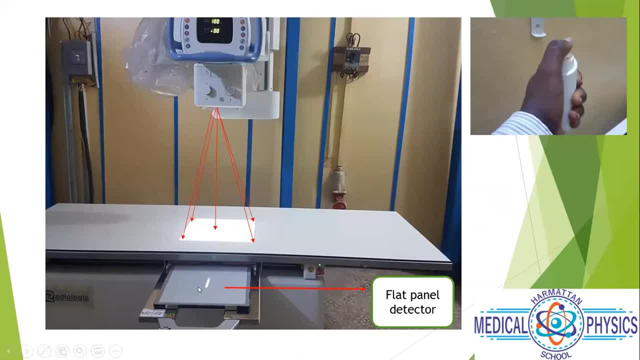 detector and on this detector. uh, we have that, this diagram. you have seen the scintillator and the photo detector, so you can actually use this. um. this is a cool metal head. um radiation emanates from here, comes out here. once i push this in, you can actually make measurement. and um in current dr system. 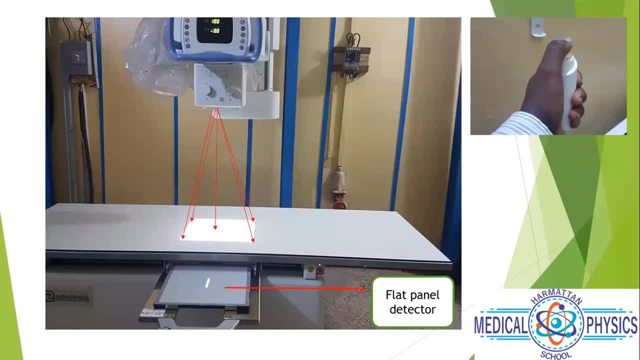 um, the flood panel system is so important that you you can use that to quantify um, your, your output, because most times in dark room process, in that room process, it's um when your image is very dark. you you should know that your factors are very high. so but in in dr system you don't really know. 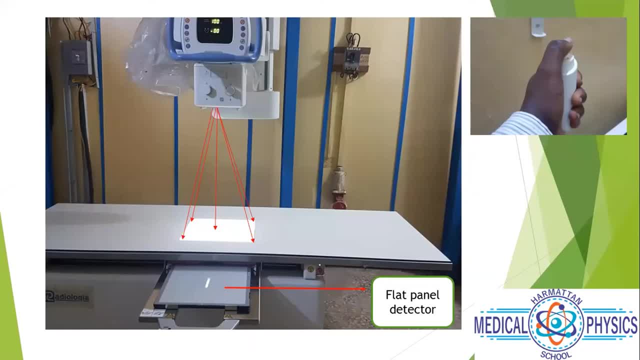 so we have what we call the current axi to actually help us measures um those incident on this flat panel system. and now for different manufacturers, we have different um? um values for you to know if um? um your output is optimal or you have over over exposed the patient. 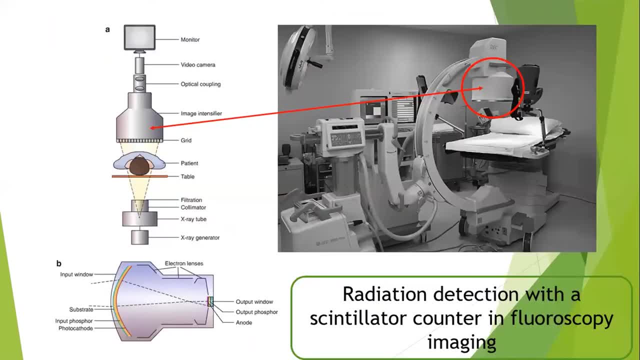 or you have under exposed the patient. so i move again to uh, a fluoroscopy system. so i- i don't know- have seen this system before. this is a fluoroscopy system. um, we, we can have them as mini uh um cm systems and usually we use them for interventional um um studies. uh, perhaps, um, you, you, you, you want. 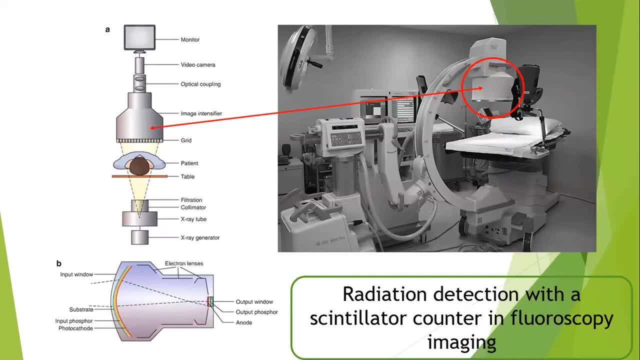 to do some um for a patient that wants to do hip replacement or femoral um. you, you want to. you, you want to work on the femur, you want to work on the tibia, the fibula, you want to work on any part of the body. so it's an image guided process. so this is actually having the x-ray generator. 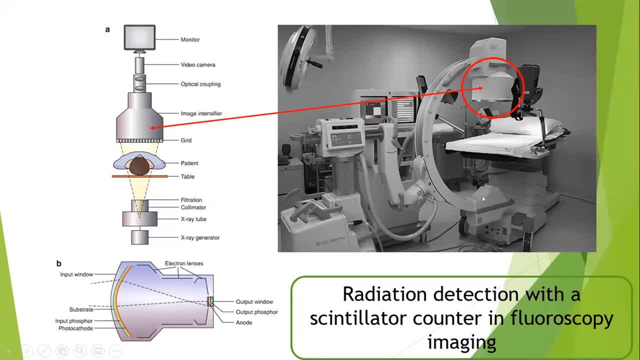 and um the x-ray tube. this x-ray tube is the same thing as this here. um, we have our um the table. yes, this is our table. we have the patient. the patient is supposed to be here now. we have our grid before the image intensifier. the grid is to help us um remove lower energy, because most times, 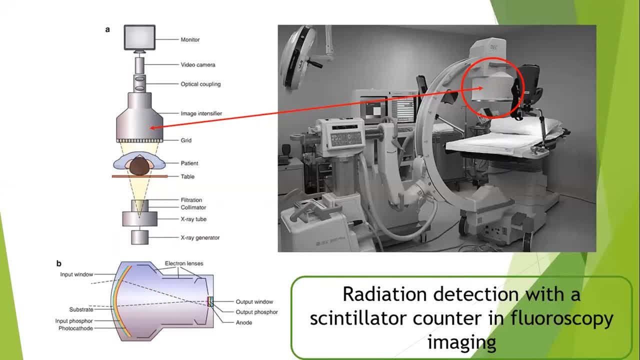 it's an x-ray and um, um photons are not, uh, uniform, like in a gamma um graph, which where energy is quite uniform, um, so these are not quite uniform, so you have to use a grid here. now we have an intensifier, image intensifier. your image intensifier has an output, phosphor. now, your output phosphor is what? 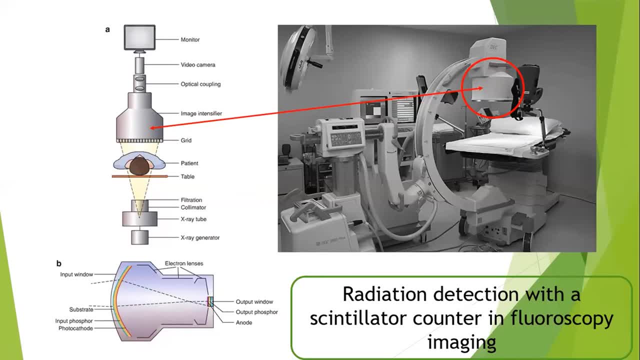 actually does the light amplification. you can see the output for phosphor is within this system and and you can actually use that. uh, there's a whole lot of light amplification. and then this time around you, you, you, you can actually use a very low dose, i mean a very low factor, to actually get significant, um, um. 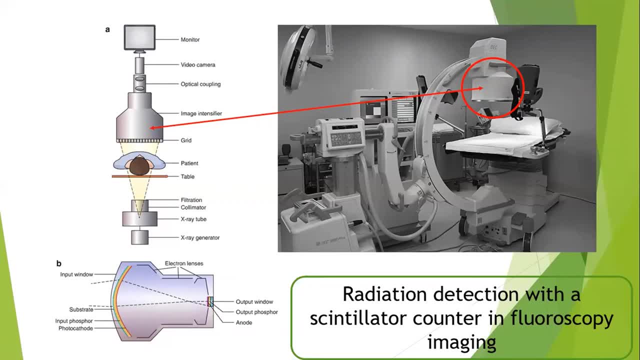 um image on your screen, practically in my center. if, if you are just um, i'm doing what we're doing. if you are just um, i'm doing what we're doing. if you are doing what we're doing. if you are just um, i'm doing what we're doing. 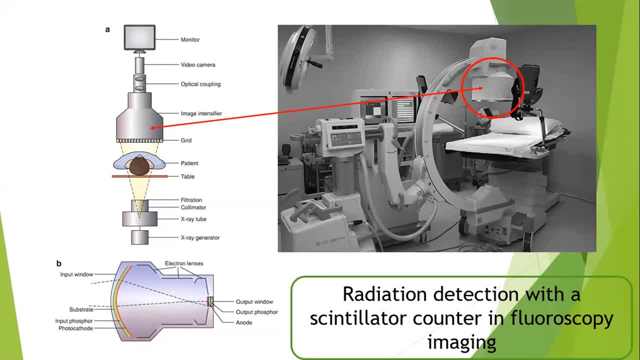 call k wiring. i don't know what. whether you know about that, k wiring has to do it. perhaps you are working on the uh, a broken arm, and you you want to try to fix them together and fixing some wires into the hand. um, you, you practically use about 43 kv, kv. 43 kv is just enough. 4 ms quite low. why. 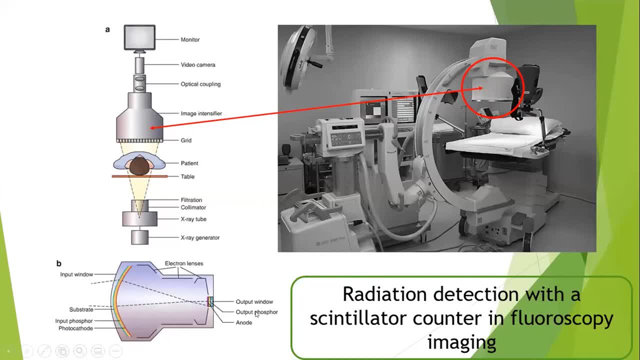 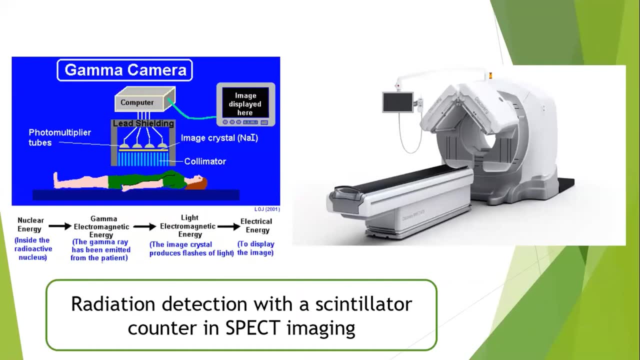 because of your output. first your output, phosphor, which does the light amplification. yeah, this is an iron unit. we call the spec imaging. that also um uses the um, um, the, the, this crystal. here you appreciate it better. here it uses this crystal and um sodium iodide, um for. 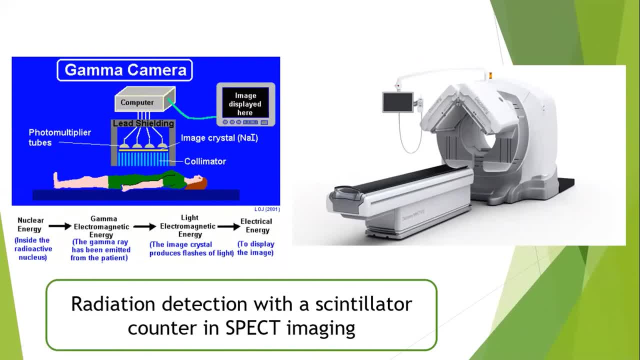 i remember our first um, um, uh i- one of our resource persons from the uk talked about this a bit and you can actually see the patient is injected with the radionuclide uh, possible technetium um 99 metastable. now we have this gamma camera closer to the patient, picking gamma rays, you have your collimator and 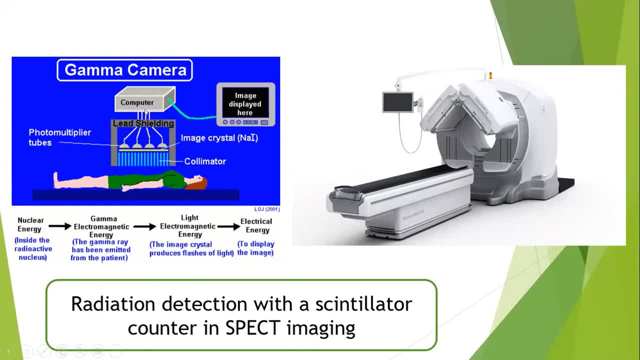 this does the light amplification, and there is a whole lot of computer manipulation and you can see images here. so you can actually use these systems and also to measure, um, those and those rays, because, just like i've said, um, the same device that can convert signals into images can also convert them into numbers, and you can actually 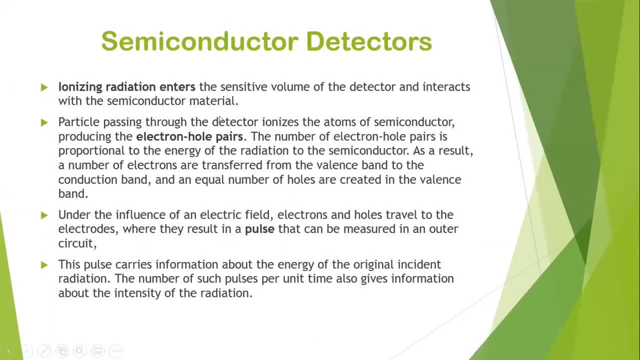 get significant results from them. i will try to look at semiconductor devices and um, um, it's quite um semixquent know скорее yet, but as we're working on this uh timeshelp video, you can also- actually this can be easily accessible on a uh near earth. uh植I could turn up a commerical facial map. uh, here can um, yeah, umuggl it or maybe yup right in the videos, so but anyway, okay, just a quick slide. you can go back and then you can see what this device is okay. okay, of course would be kind of a Mingle. you maybe have that. uh, your hands are on a fiberglass, or have a itsi you before contract. 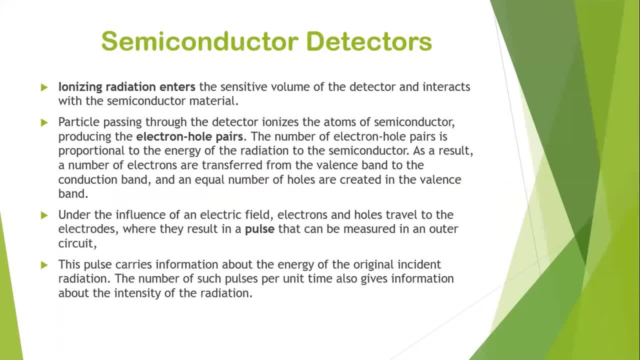 but it's you also. you can see, i can just fill that falls and try to put some things in it, and then you also need a video to show you. semiconductor device is quite um for us. that did solid state physics i. i know you are going to remember your bravia lactis, your um three, two one. is it three two, two one where you 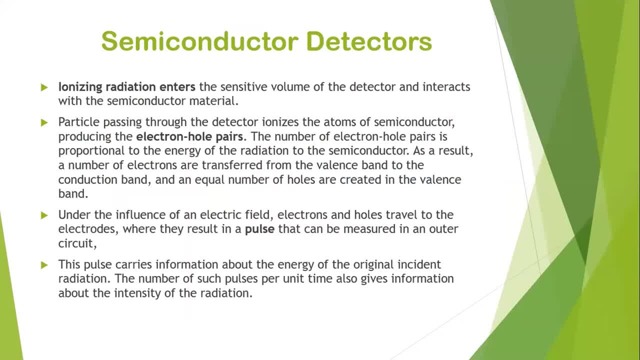 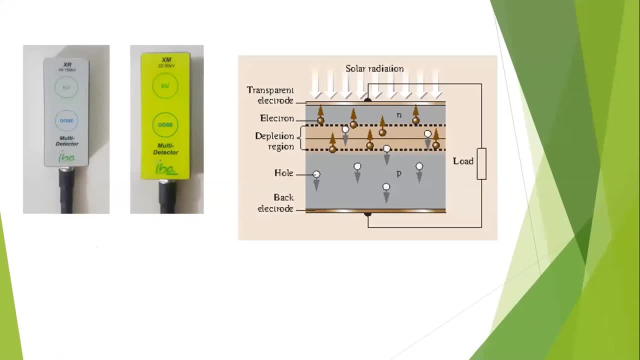 draw your brava lactis and then you try to: yes, it's, they're all semiconductor devices. uh, practically i have an image of a semiconductor device, um, which i use um for measurement of those. those reads me, ms, several parameters. so it's quite amazing. now, this depletion layer. 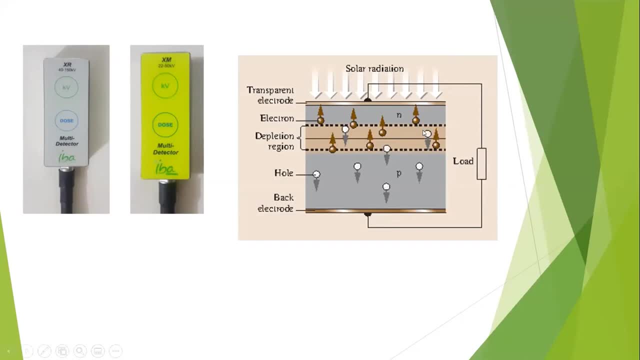 is actually where there is reionization. reionization takes place here, and then there is: you can actually get your, you can actually get your dues from here, you can actually get your parameters from here. so i'm i i know i'm quite running out of time, i have to just um, hang it up here. 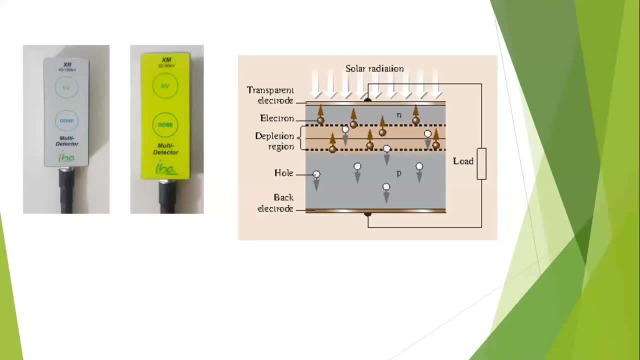 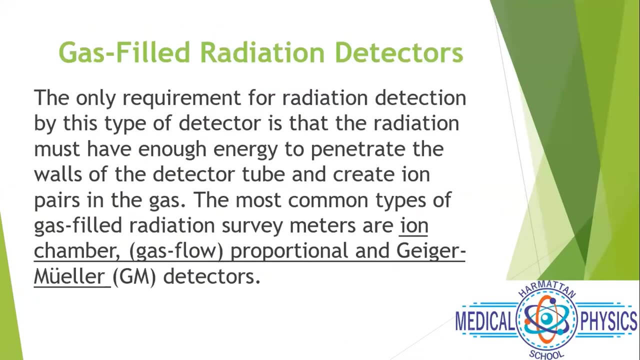 thank you very much, uh. i i don't know if there are questions. if there are questions, you can do well to ask me questions. i'm ready for that, all right? thank you very much, uh, mr modular.